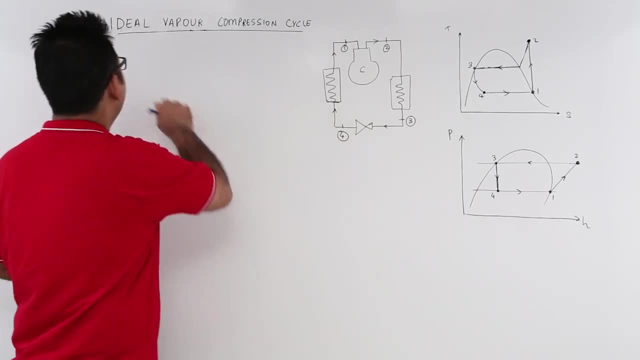 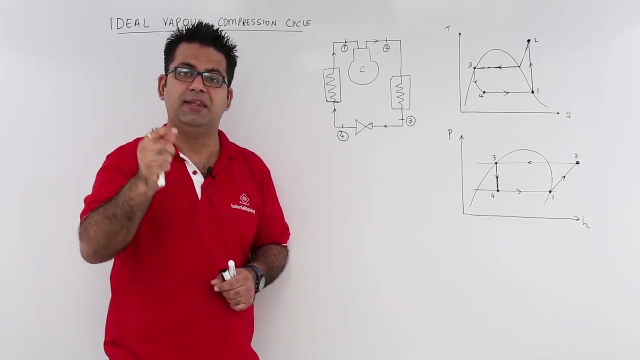 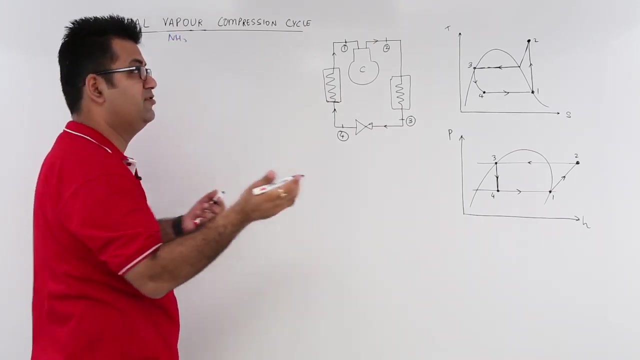 Now, in this video, we will start discussing about the ideal vapor compression cycle. In the previous videos we looked at the air refrigeration cycles, in which the working fluid was air, But in this we will be using some vapors of gas. Now that gas could be ammonia, that gas could be any gas. You can have CO2 also. 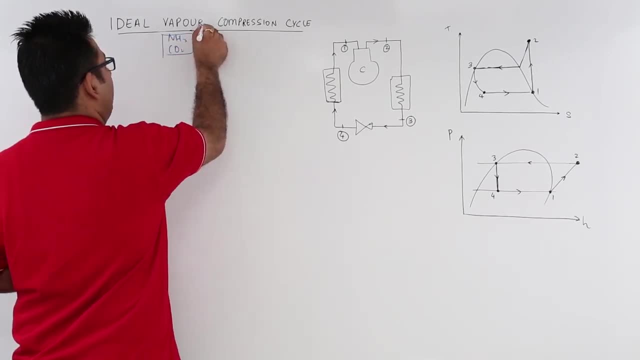 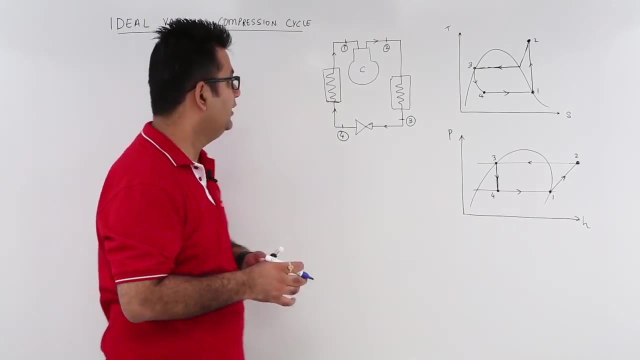 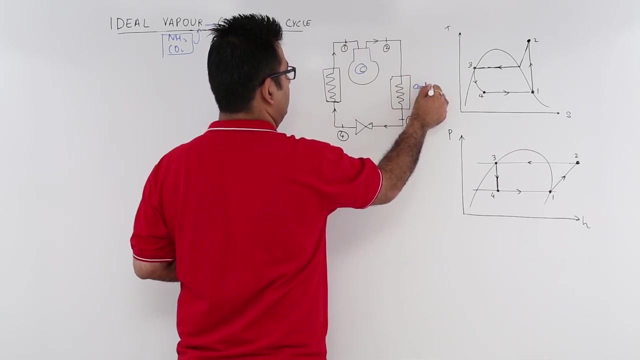 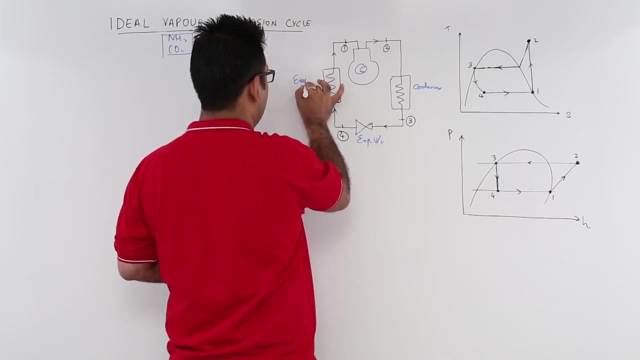 So any gas and its vapor will be compressing those vapors to create the cooling effect or the refrigeration effect. The schematic stays the same: You have a compressor, you have a condenser, you have an expansion valve and you have an evaporator. 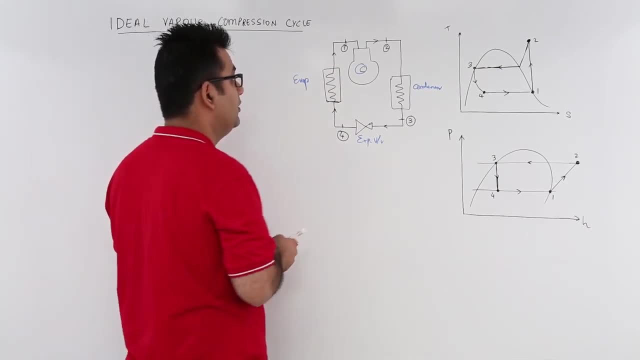 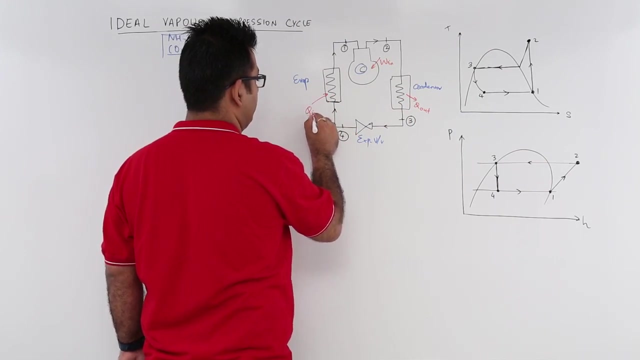 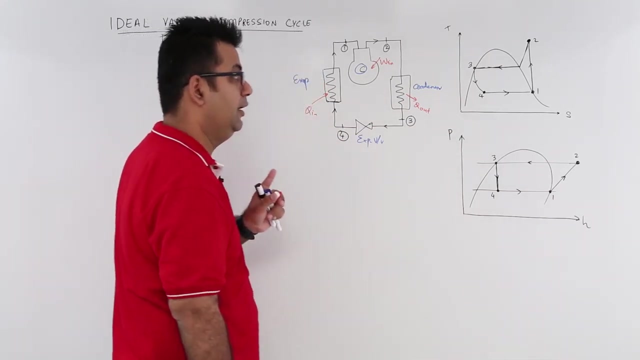 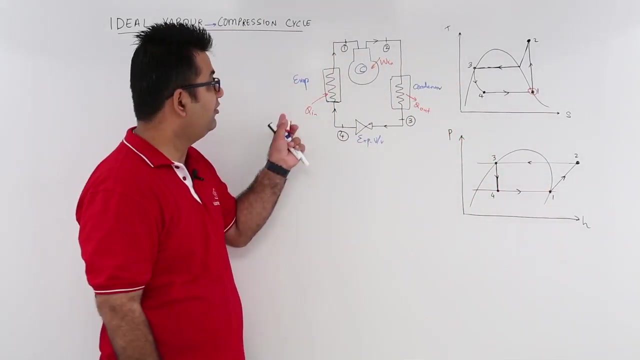 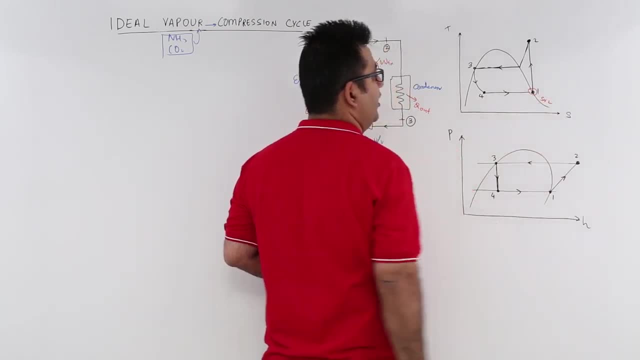 Okay, If you look at the TS and the PH plot for the ideal compression cycle, it is always assumed that the vapor enters the compressor after the evaporator see it is on the saturated vapor line and also in the pH plot. this is the point at which 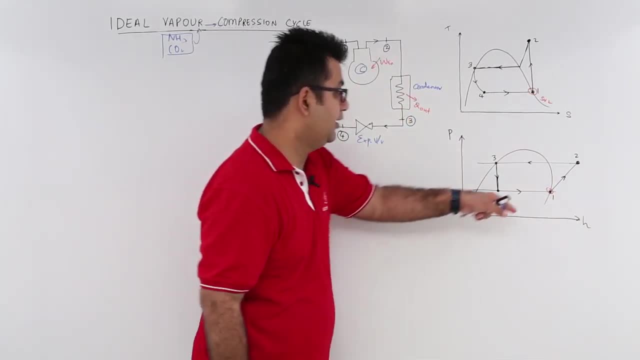 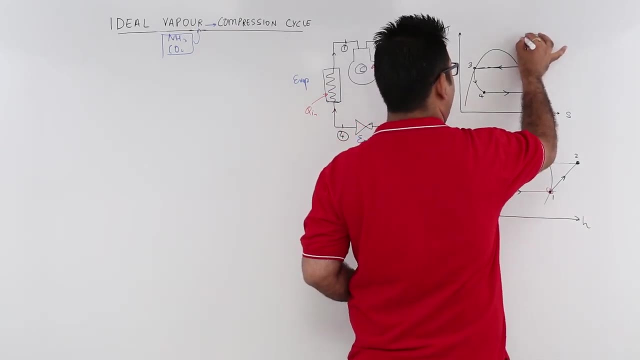 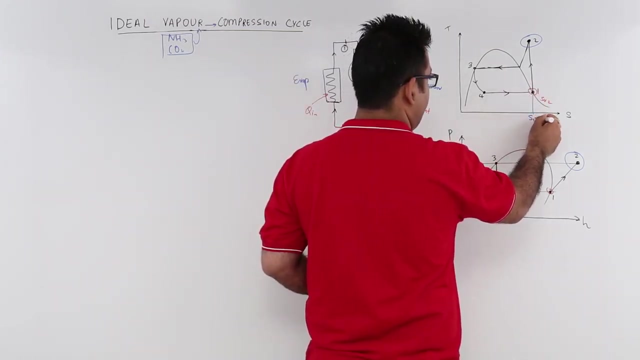 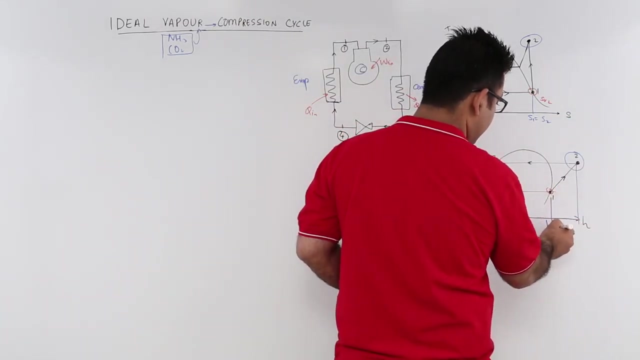 the vapors enter the compressor, that is at the saturation point or the saturation condition. after compression, the vapors attain a superheated state at 2. ok, so this shows you have an isentropic compression and this shows that upon compression there is an increment in the heat value, that is, 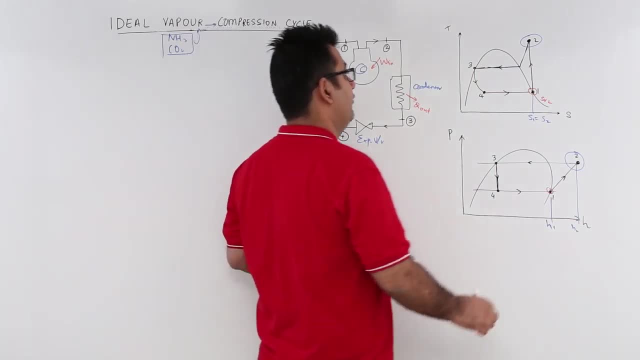 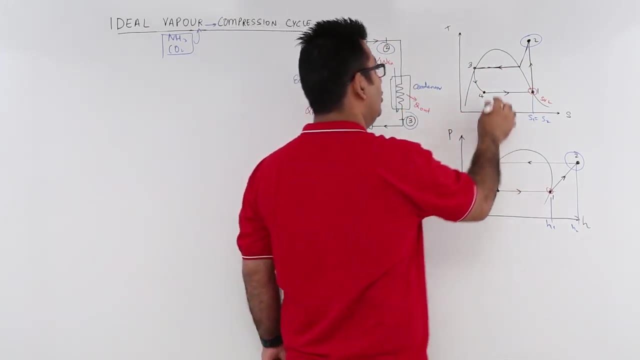 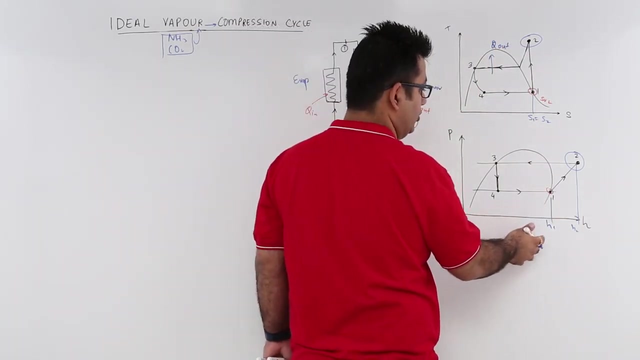 the enthalpy has gone up now from 2 to 3. 2 to 3. you are going through condenser so you lose some heat to the surroundings. so this is Q out. ok, and this is evident from this diagram also, that your enthalpy 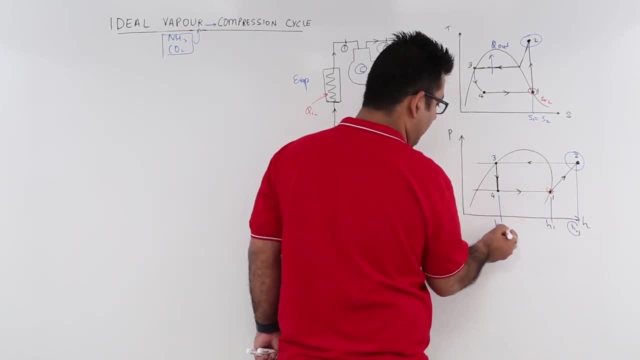 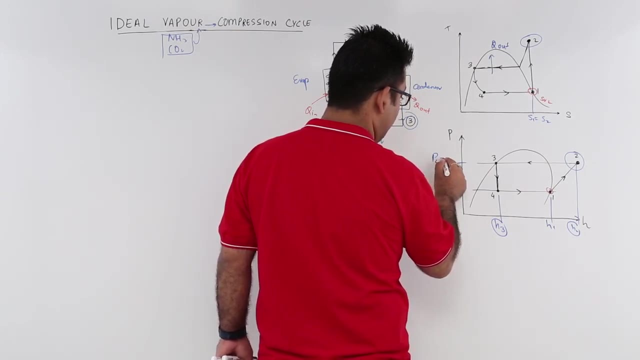 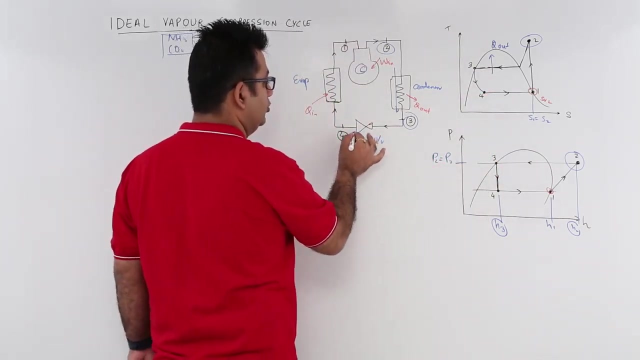 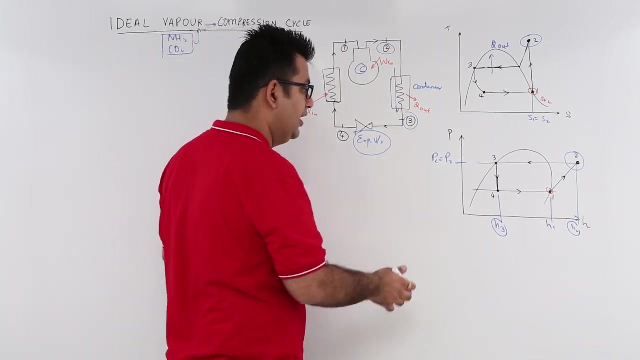 drops from H2 to H3. ok, so you lost some heat, but at constant pressure. ok, now from 3 to 4, that is, you go through the expansion valve. now we assume that during this expansion valve the enthalpy remains the same. the enthalpy remains the same, but there is an increase. 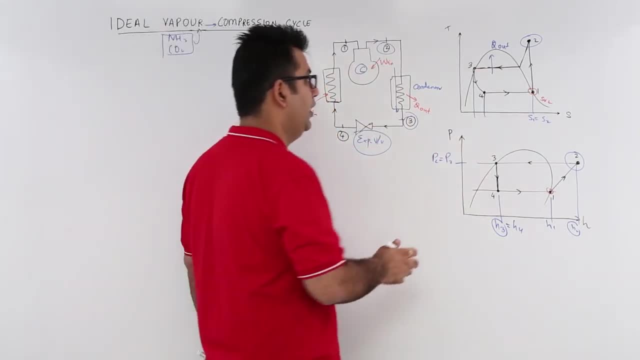 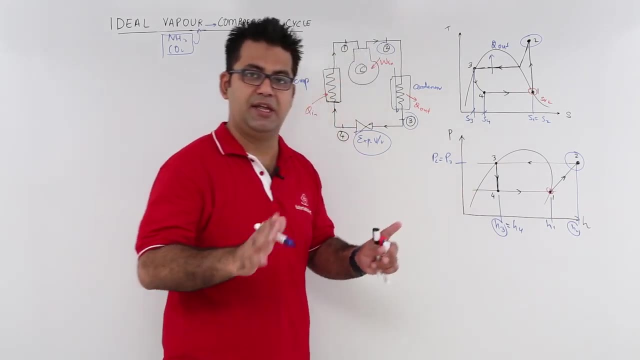 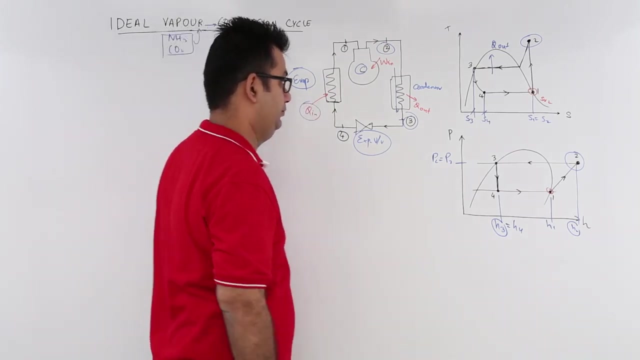 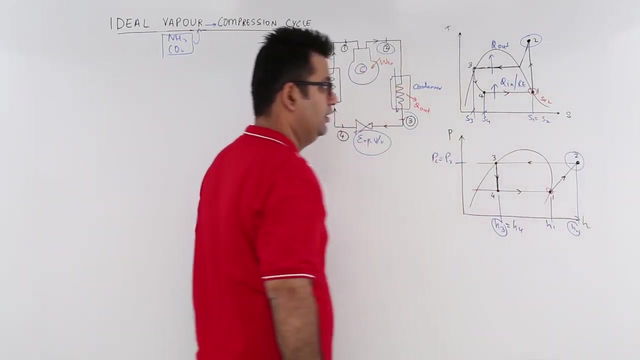 the entropy, because the expansion is taking place. ok, so this is s3 and this is s4, but the enthalpy is same. now, from 4 to 1, you have to go through evaporator, so there will be some heat input. so 4 to 1 is q in, or it is also known as the refrigeration effect, and 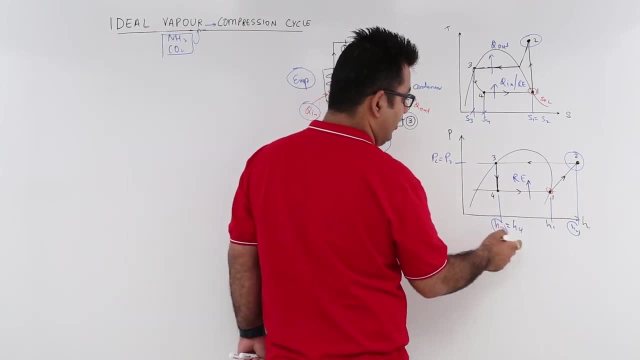 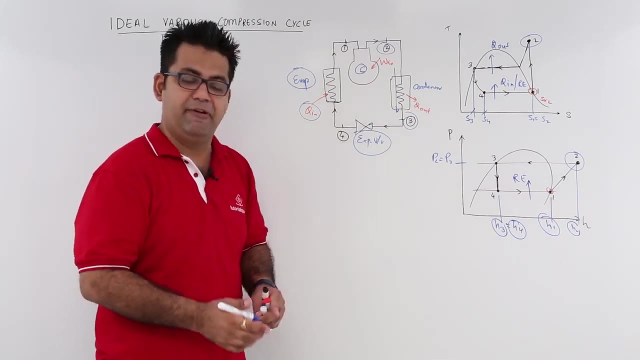 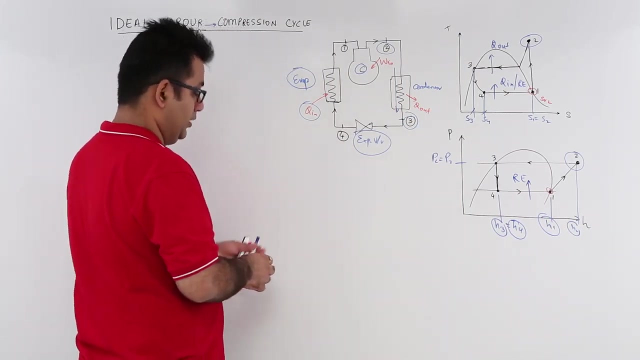 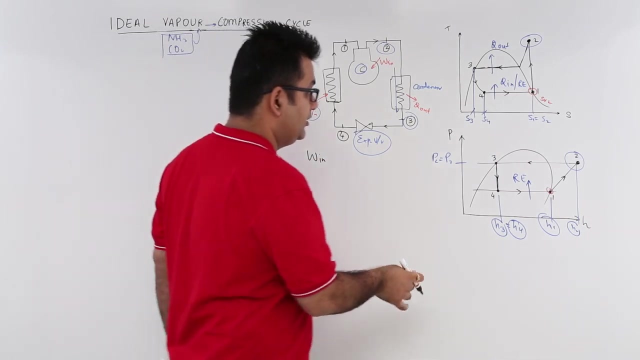 this is the Re and you can see that your enthalpy increases from h4 to h1. so this is the ideal vapor compression cycle. now let's analyze it for work input and COP of the cycle. so if you find out the work input per unit mass, ok, let's take the enthalpy values only, because 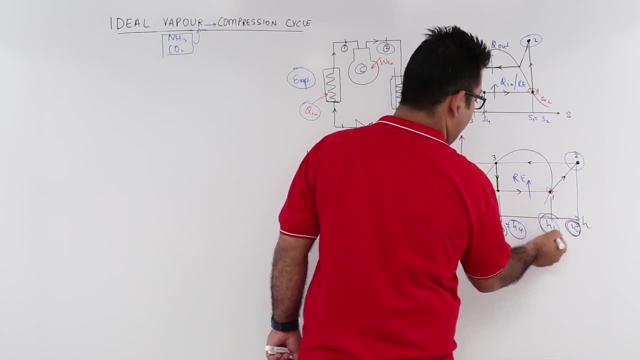 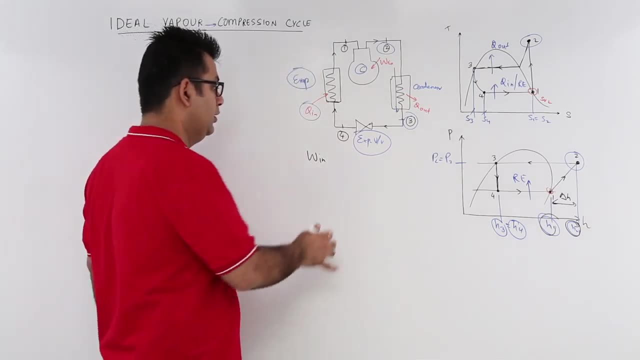 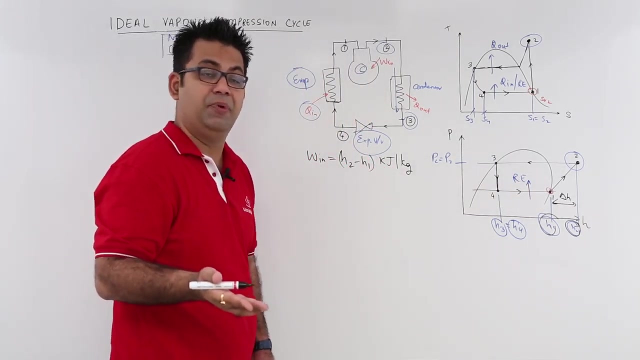 they are easiest to take. you have h2 minus h2, and this is the vapor compression cycle minus h1. this much is the energy input in the compression cycle. so you will have h2 minus h1 kilo joule per kg. ok, now the refrigeration effect, because we just need 2 things for COP. 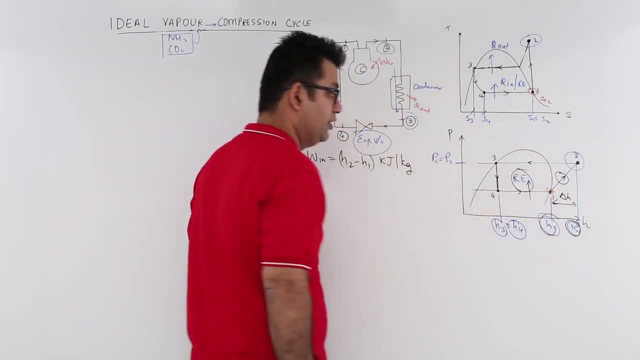 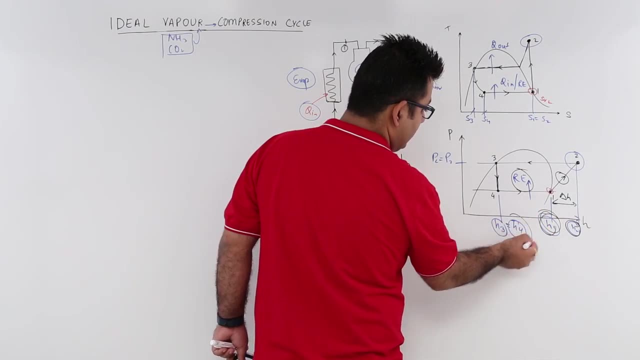 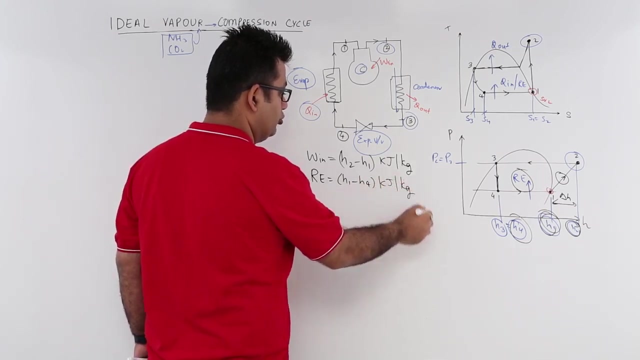 we need the work input and we need the refrigeration effect only. so the refrigeration effect is given as entire body and theロ neither is equal to either of it. it will give you the work input, as I told you, the difference in these two GRANT help. you will have h1 minus.